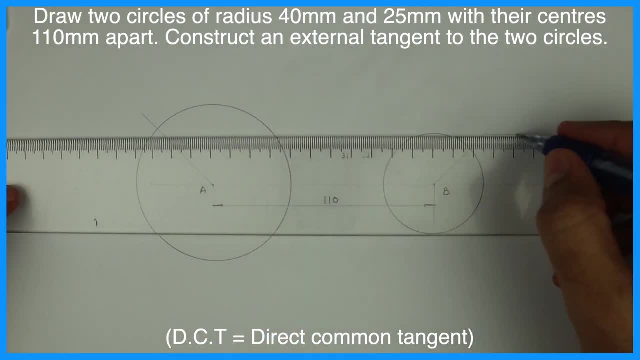 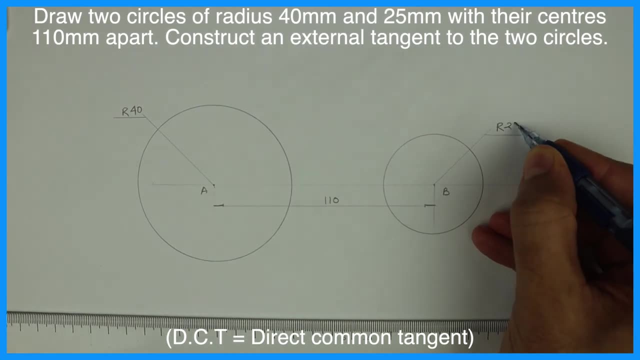 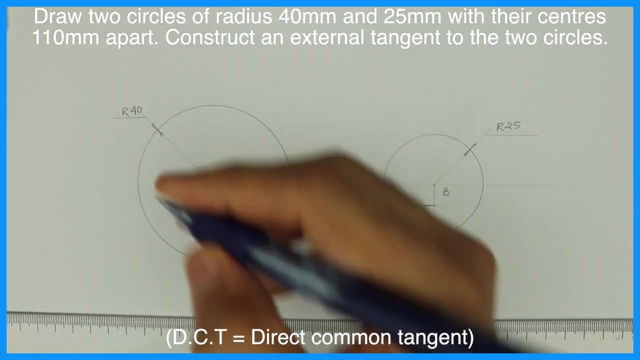 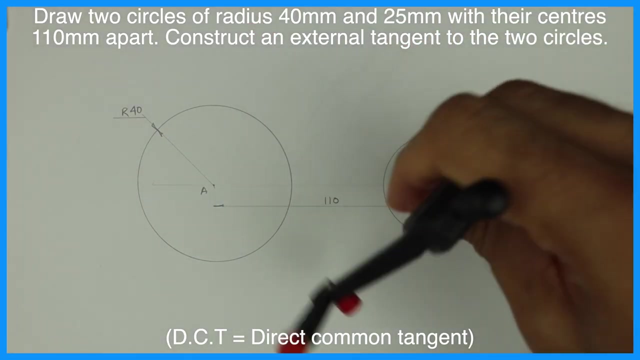 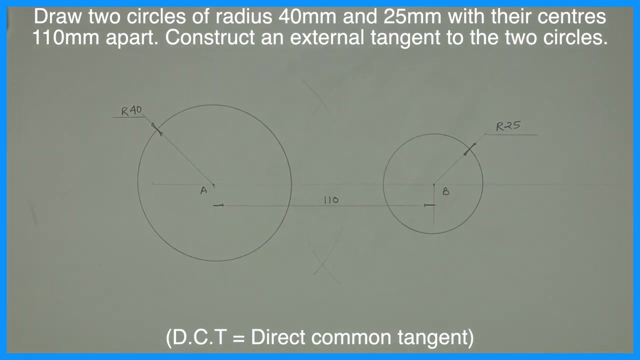 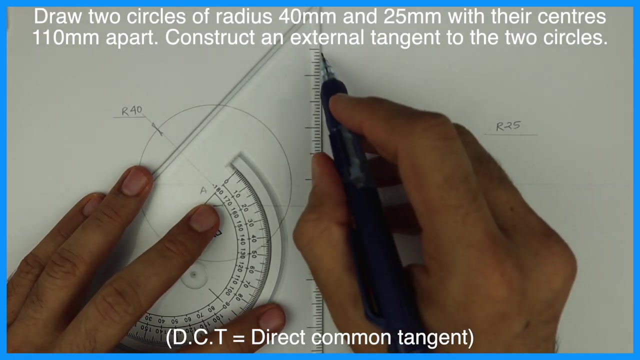 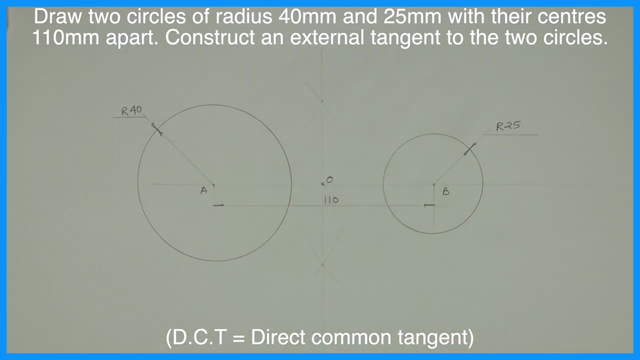 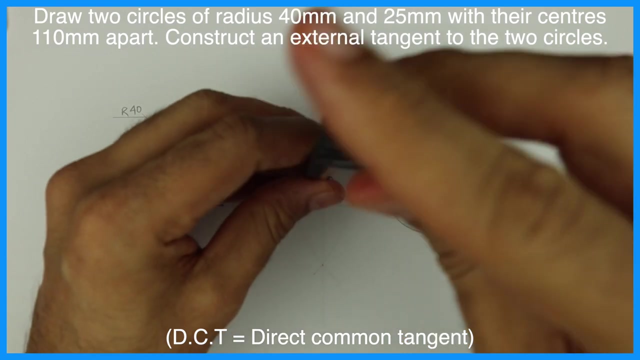 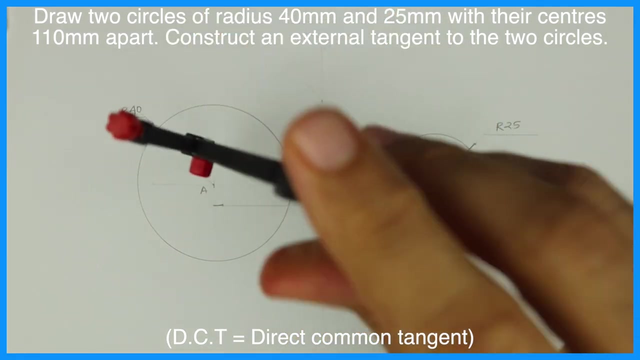 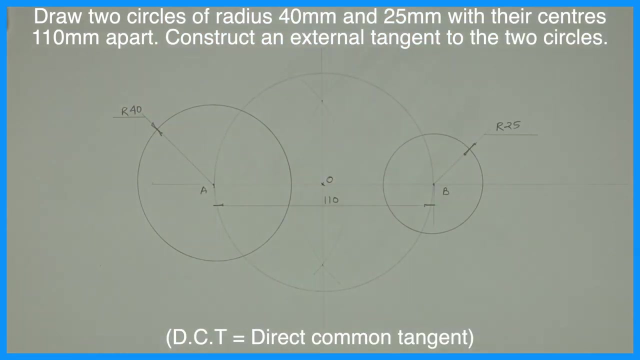 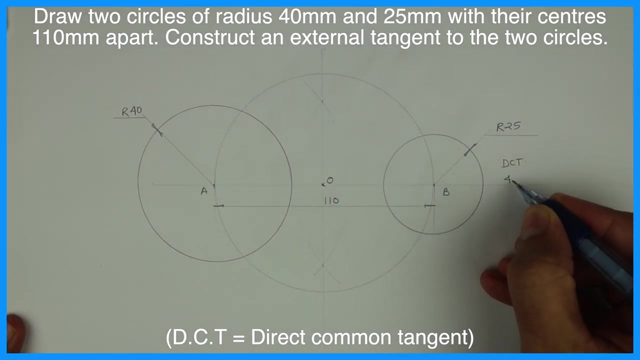 This is radius 40,. this is radius 25.. Then you bisect AB, You mark that point as O. Now take O to A and draw a circle. See this: now we are drawing DCT. So what I remember as DCT is deduct. 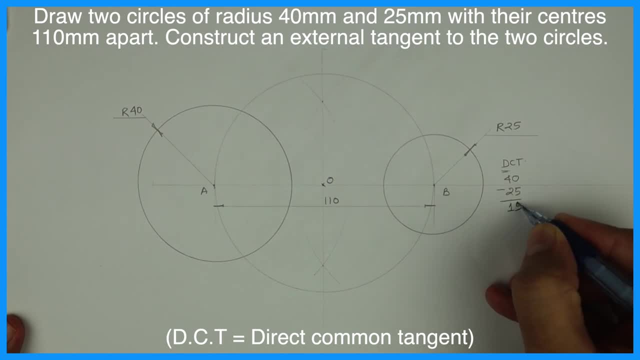 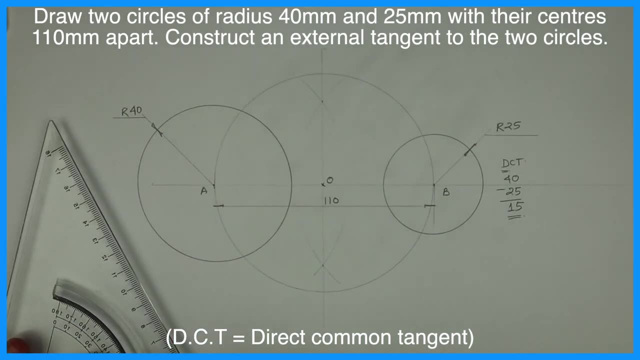 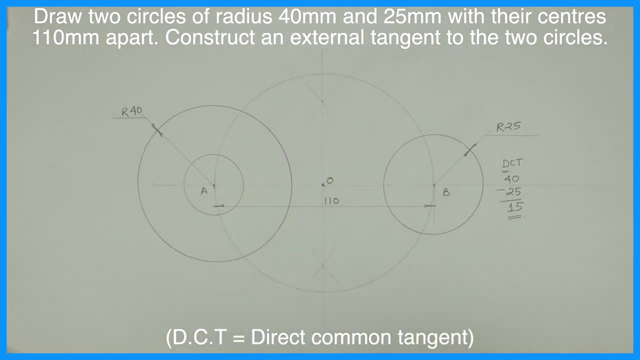 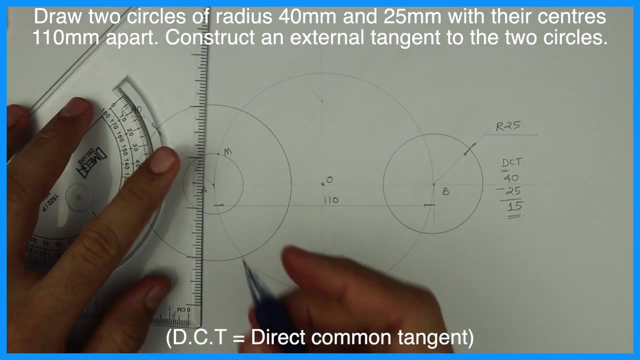 So I'll do 40 minus 25, the bigger radius minus smaller radius, I'll get 15.. So I will use 15 mm radius from A. See this from A. I will draw radius 15 mm And I will get that point as M. Then I will join A to M. M is the point where it is intersecting. 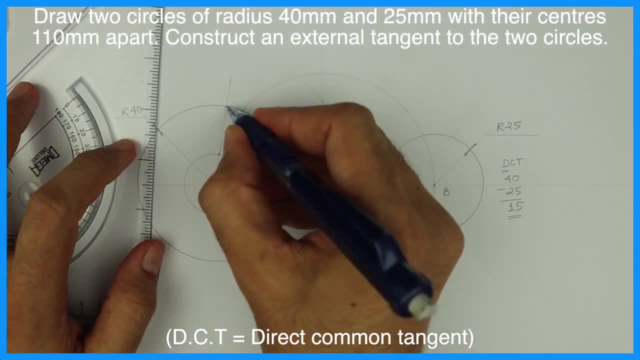 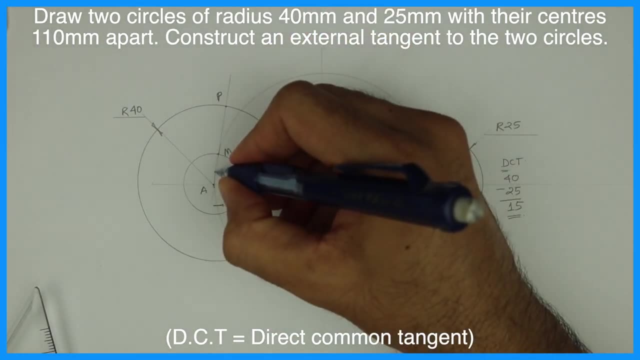 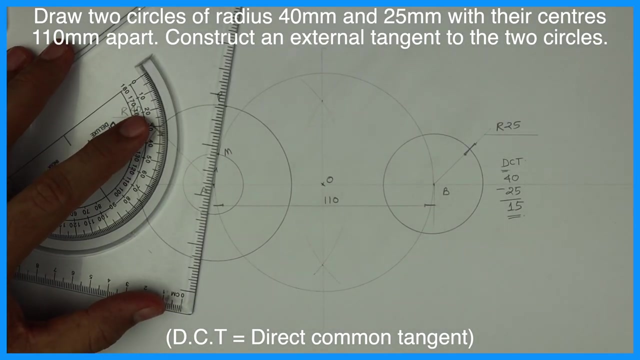 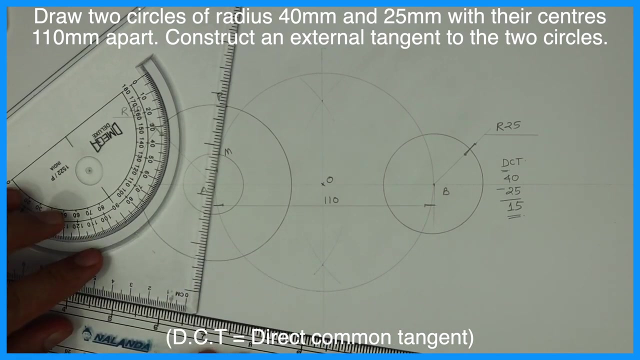 with the middle circle, that bisector circle, And then extend A M wherever it will cut. that is point P. Now we need to draw parallel line to A P. See this. we'll keep side square like this. We'll keep a scale below. 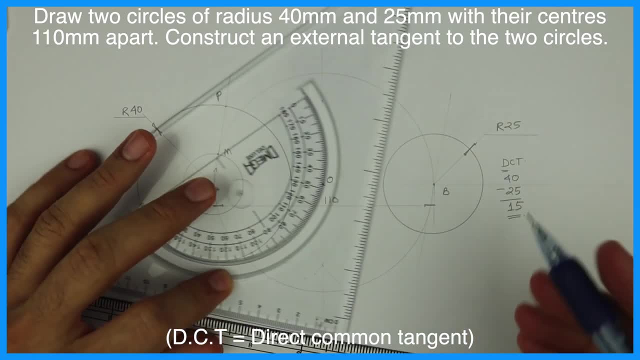 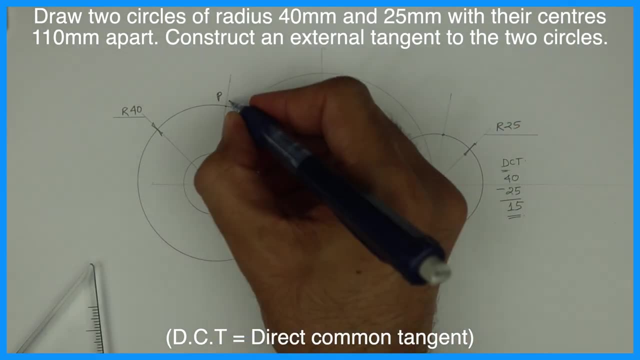 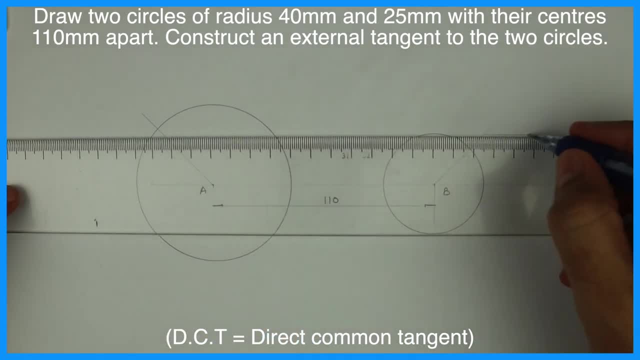 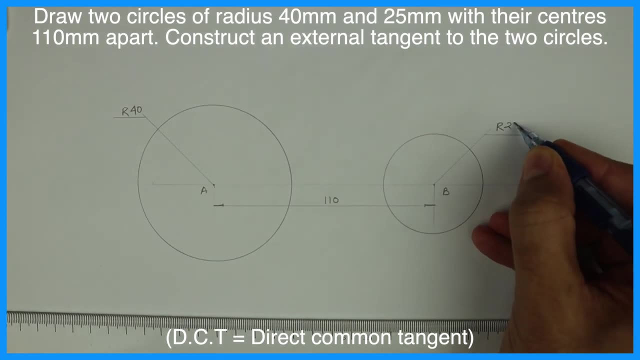 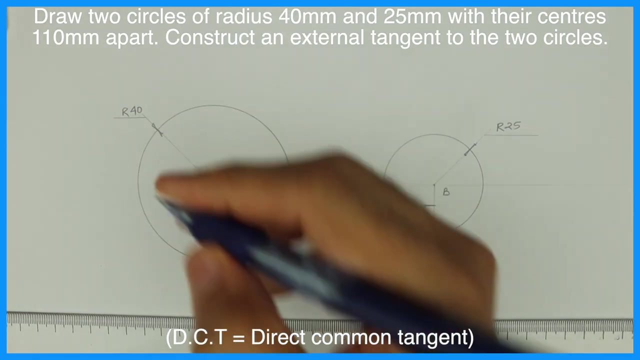 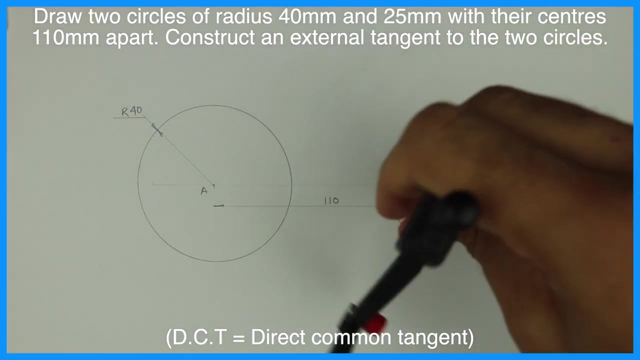 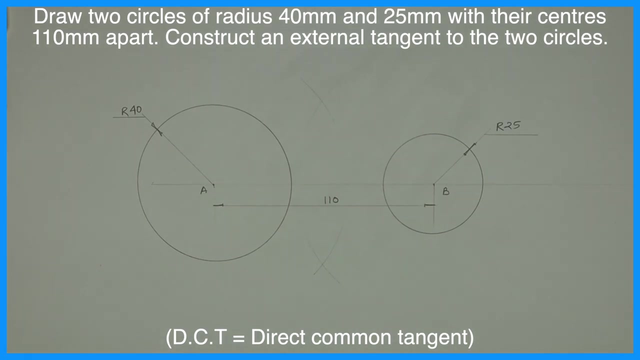 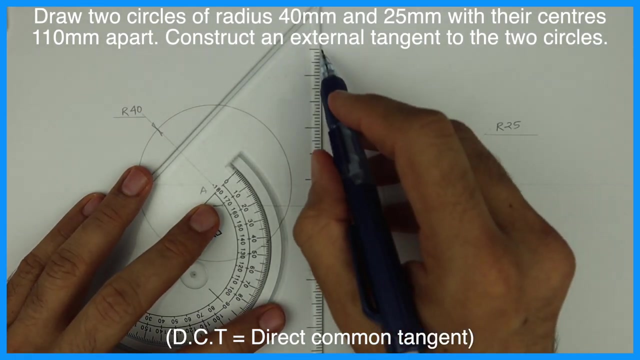 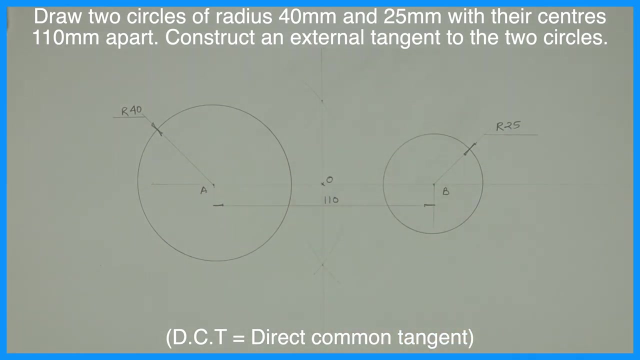 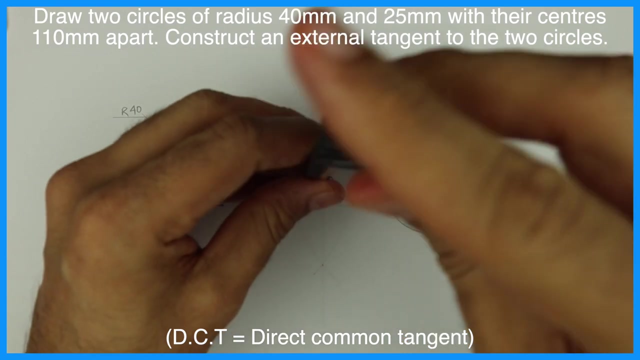 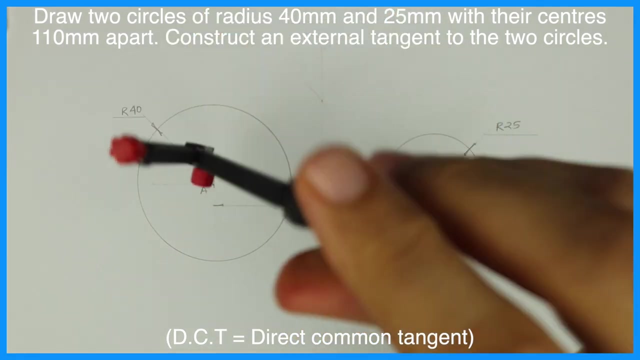 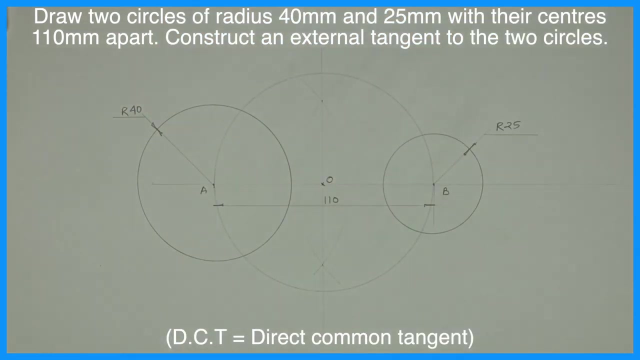 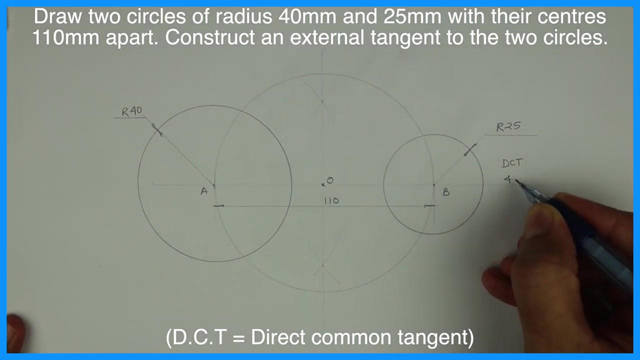 This is radius 40,. this is radius 25.. Then you bisect AB, You mark that point as O. Now take O to A and draw a circle. See this: now we are drawing DCT. So what I remember as DCT is deduct. 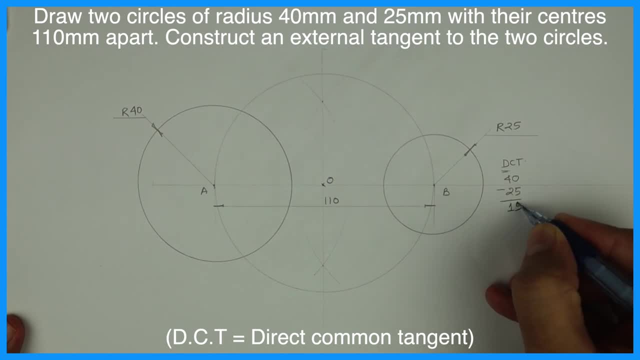 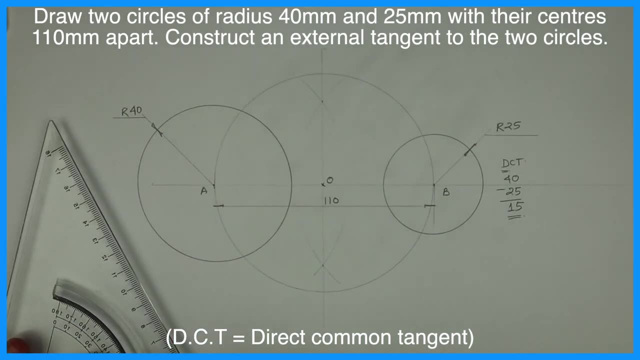 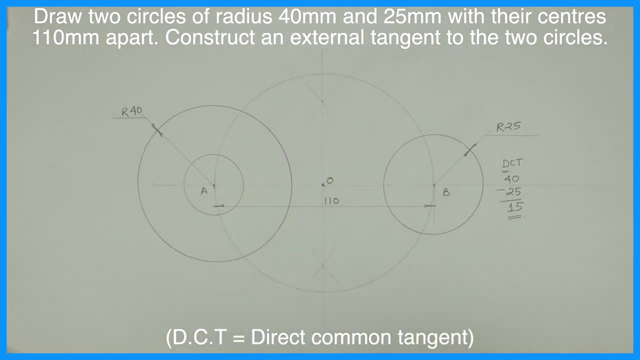 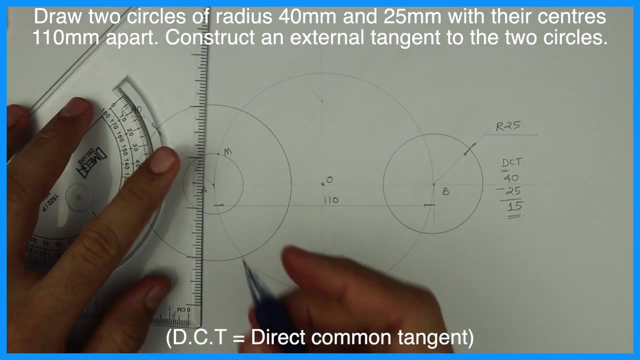 So I'll do 40 minus 25, the bigger radius minus smaller radius, I'll get 15.. So I will use 15 mm radius from A. See this from A. I will draw radius 15 mm And I will get that point as M. Then I will join A to M. M is the point where it is intersecting. 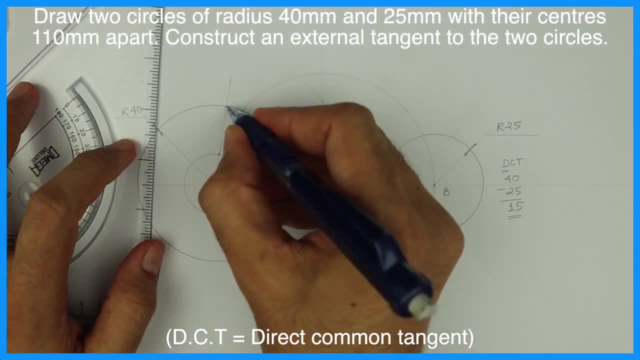 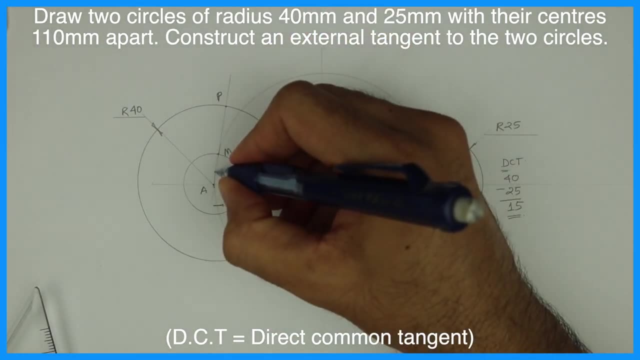 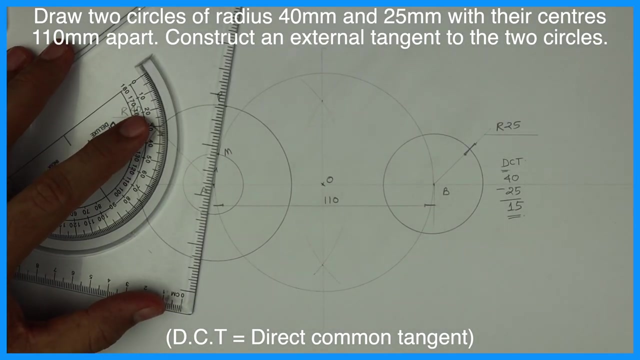 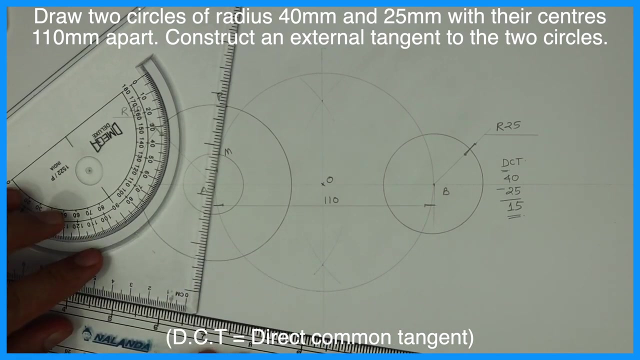 with the middle circle, that bisector circle, And then extend A M wherever it will cut. that is point P. Now we need to draw parallel line to A P. See this. we'll keep side square like this. We'll keep a scale below. 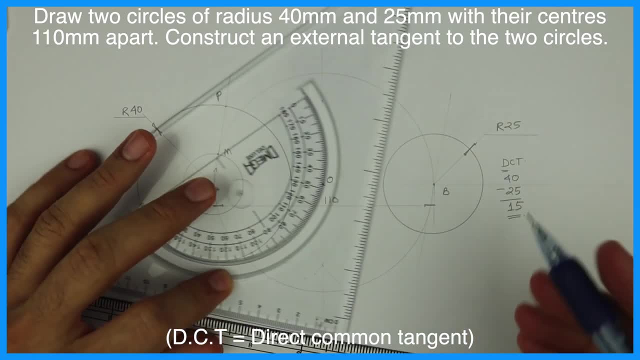 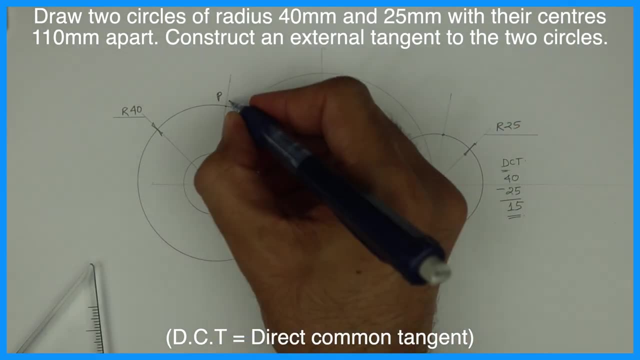